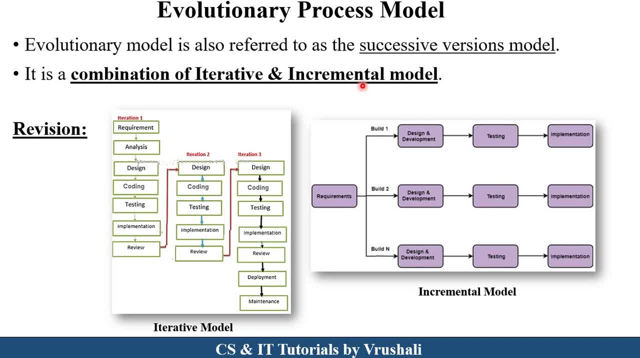 We already discussed iterative and incremental model. So what's the purpose of iterative and incremental model in detail in previous session? Here we just take a revision of this model first. Now what exactly iterative model we will discuss in this diagram Here. in first iteration they collect the requirement from the customer. 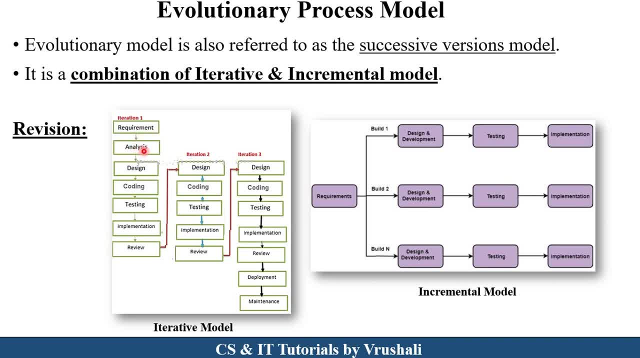 After collecting the requirement, the analyze those requirement And after requirement analysis they design, code, test, a complete product. After completing the implementation Then they idealize어� cause ease of model development. in this section review from the customer. if customer want any changes, then they again move to second iteration. 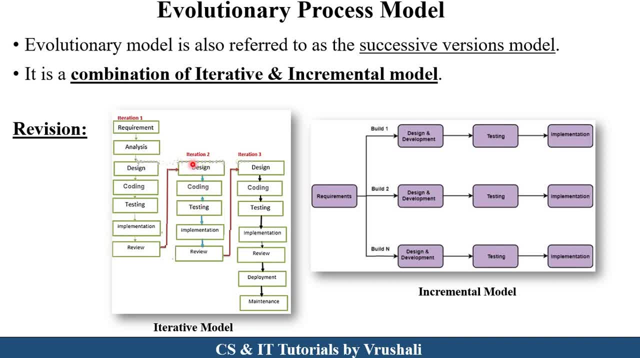 that is again the design code and test the product after complete implementation. they again take a feedback from the customer. if customer want any changes, they again move to next iteration. again they design code, test a complete product. after that they again take a review from customer. if customer want, all okay, then they deploy the product to the customer. 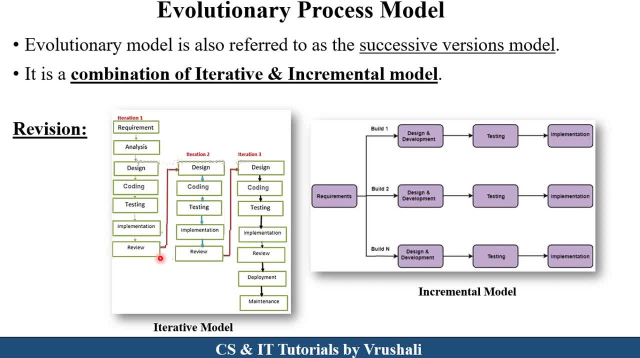 this is the concept of iterative model means they develop a product iteration wise, and after completa implementation of product, they take a review or feedback from the customer. okay, this is called as iterative model. now, what is incremental model? in incremental model, they didn't develop a complete product at the same time. 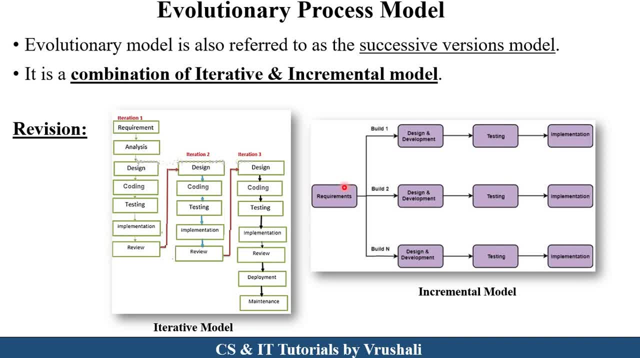 they first gather all the requirements from the customer and this requirements are now freeze. after collecting this requirement they divide those requirement into the multiple modules. here, module by module, development is in incremental model. we discuss example of college management system. suppose customer want college management system. so after gathering requirement first they develop attendance module. they 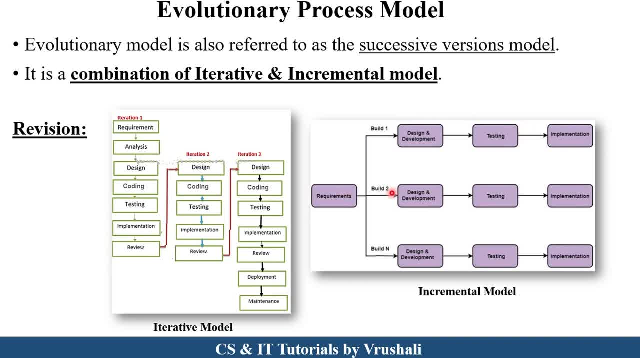 design, develop test the module. second, they want feedback module. they design, develop test this module. and third, they want teacher module. they again design, develop test. this module means here every module come from design. development. testing means complete software development lifecycle, right and after completing this complete product, then they take a feedback from the 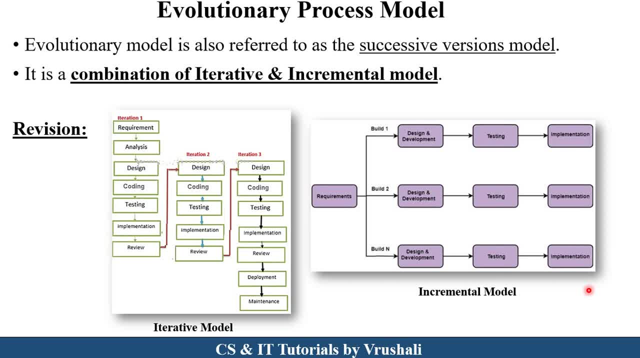 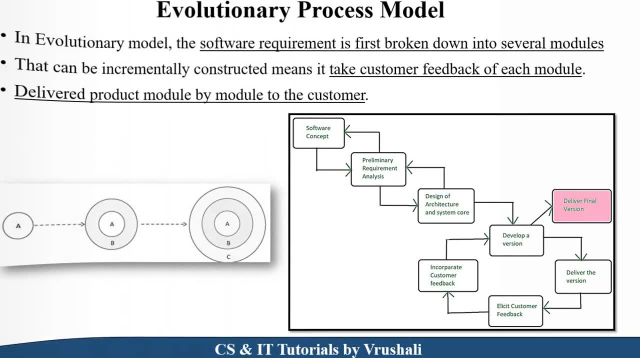 customer right. so this is a incremental model. now evaluation easy process model is a combination of both house the next c here in evolutionary process model, the autonomous rocks, Kovalo missionary process model. okay, here shows software development life cycle start and the forced visit requirement announced past the customer called management system. 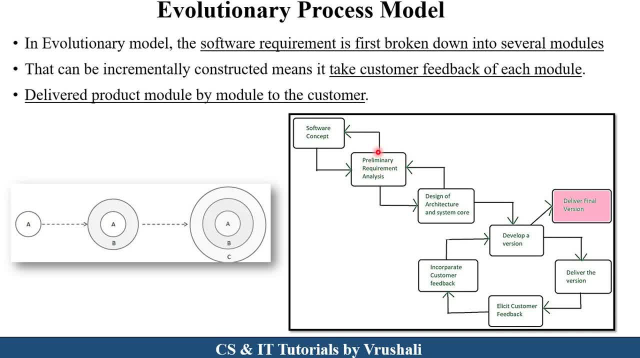 project project, if that they collect all the requirement request point from the customer. right now they divide those requirement into the multiple modules. so first module is suppose attendance module. they design a attendance module. after that they develop attendance module. that is a first module or first version. we say right after developing. 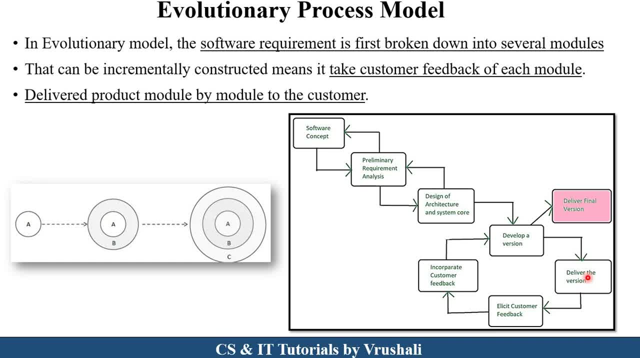 a first module. they deliver this module to the customer. now, customer get a feedback. they take a feedback from the customer. If customer want any changes in attendance module, they again redevelop it or re change it and after that deliver the final version to the customer. similarly, after first. 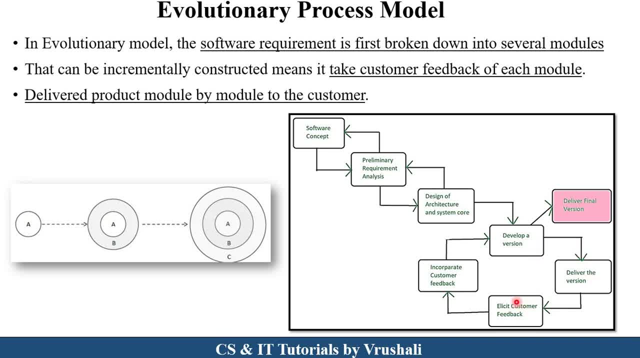 module. level them please- those student feedback model to the customer. they get a customer feedback. if customer want any changes, then they redevelop it, rechange it in this particular module and deliver the final version of the module in this way. so what is in evolutionary process model? first, they divide all the requirements into the modules. second, they develop all the particular product module by module. okay, and after each module they take. 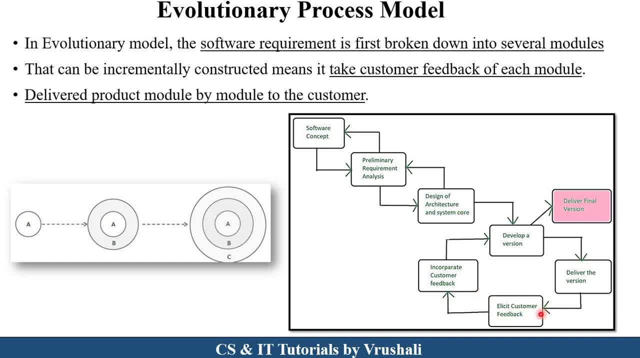 a feedback. this is a extra thing which is not available in iterative and incremental model. okay means after every module development they take a feedback from the customer. if customer want any changes, they redevelop it and deliver the final version. so this is called as evolutionary process model. see here in this image. suppose this is the first A. this is the first feature in this module in the project. like first module is attendance module. after 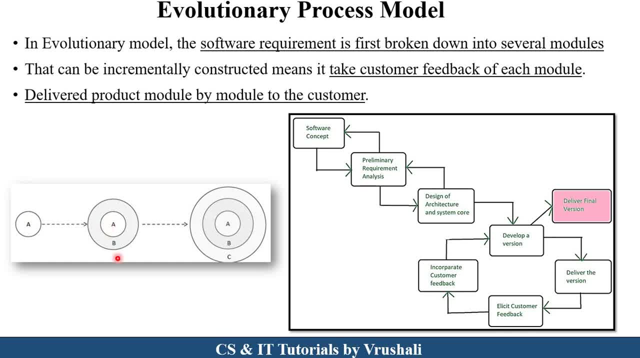 that they deliver to the customer after customer wants to run feedback module- that is B- then they deliver complete module to the customer after that customer want third feature, that is teacher module, then they deliver this module to the customer. so this is the incremental approach and this is the iterative approach. means every module they take a feedback right. so this is called as evolutionary process model and that's why it is called as successive version of module. 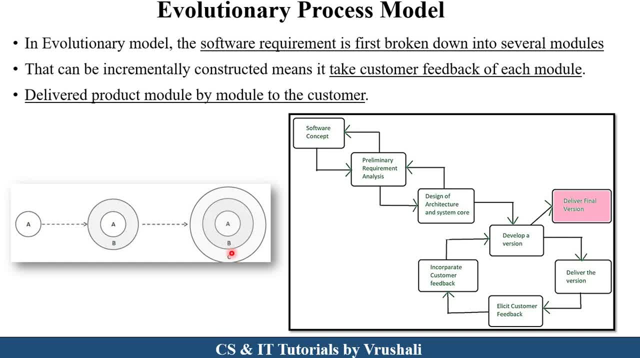 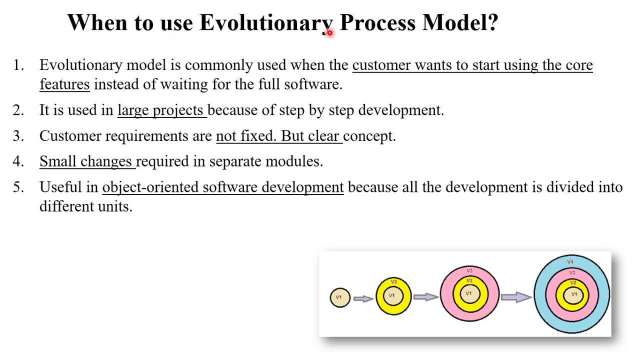 it has a better accuracy as compared to iterative and incremental model. clear next now. the next is when to use evolutionary process model. first, evolutionary process model used in large projects because here is a step by step development of particular project. the second thing is here customer didn't want a complete product. at the same time, customer get the product. 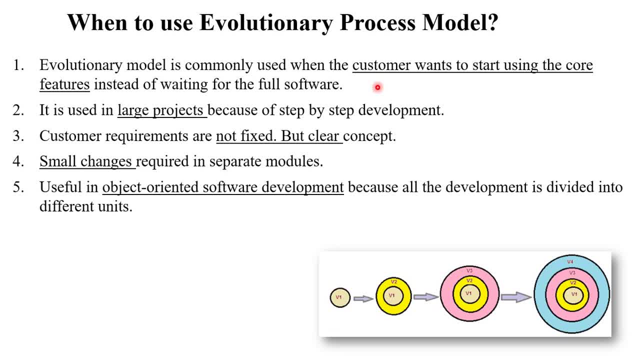 as per their priority, as per their usefulness. suppose a particular organization priorities attendance module, they need attendance module quickly, so first develop it. second, they want customer student feedback module. then develop this module in this way means customer want to start using the core features instead of complete full software right next. in evolutionary model customer requirements are not fixed because after every 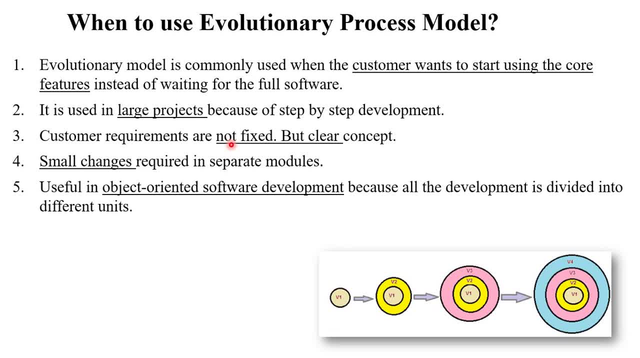 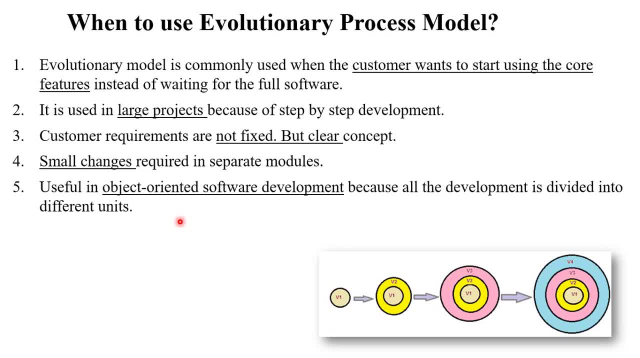 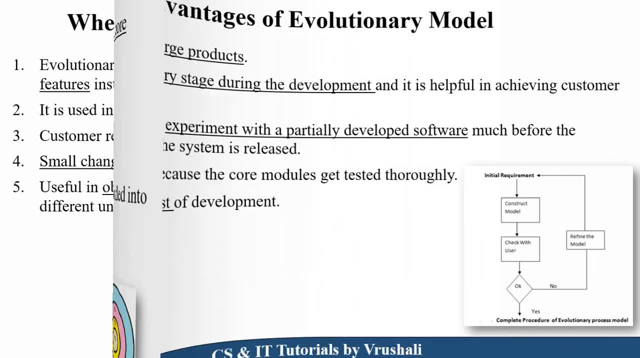 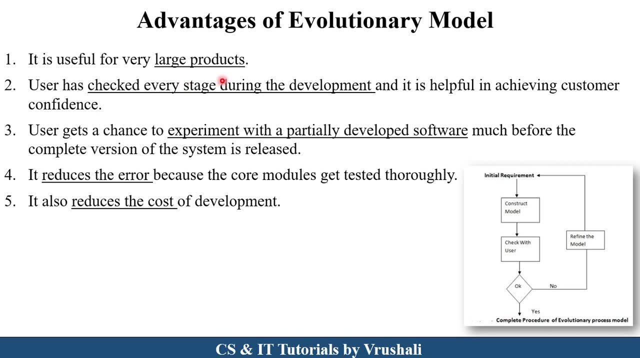 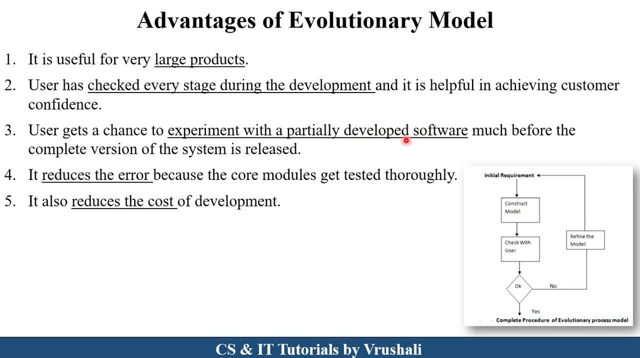 is: user get a chance to experiment with partial develop software right. user can't wait for fully version of particular software. next, if it very easy to reduce the error- because you need to solve the error in particular module, not a complete project, and it also reduce the cost of development. see, here this is a just a concept and that's why this is. 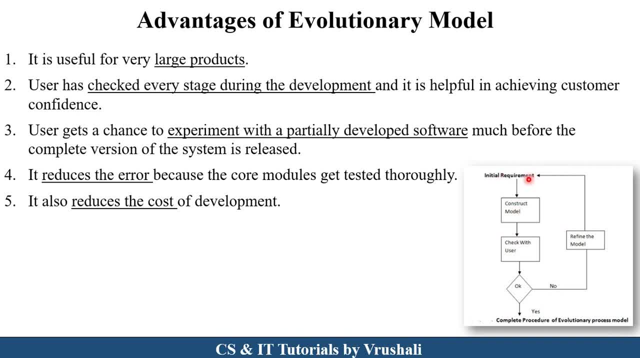 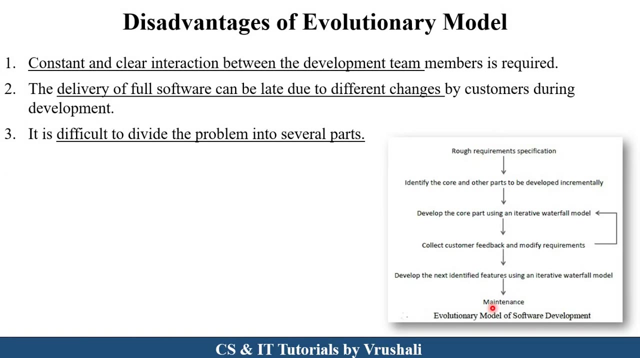 the advantages of evolutionary model. first, initial requirement. then construct the model. check with user. if customer want ok, then develop a second module. if customer want not ok, then they find the module again, construct the module in this way. so this is a flowchart of evolutionary process model. next now, the next thing is disadvantages of evolutionary model, here constant and clear. 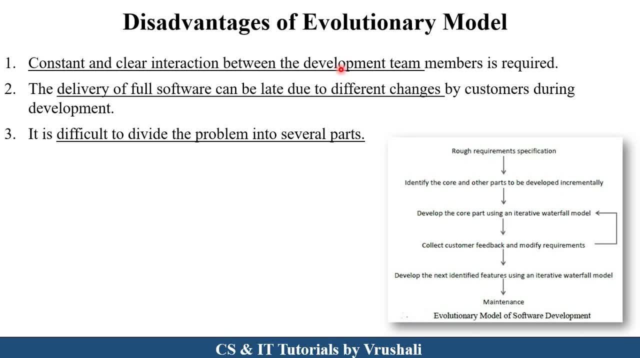 interaction between the development team is necessary means there are lot of customer interaction. after every module they take a feedback from customer, so it take a some lot of time in some what projects right. so constant and clear interaction between development team is necessary here. the next thing is delivery of full software can be late due to different changes because 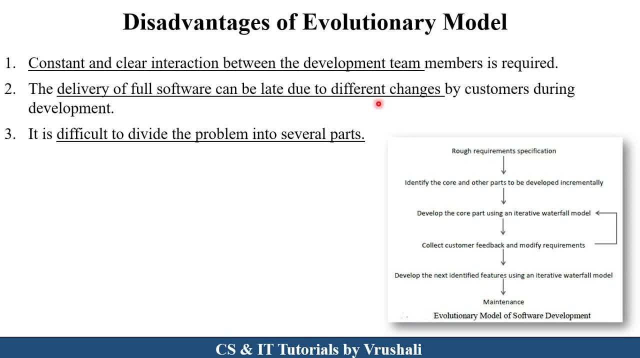 suppose each and every module customer want changes, so delivery of product is being late, right. next thing is it is very difficult to divide problem into the several parts. see, some projects will be very complicated, right. so sometimes it is very difficult to divide the particular product module by module. so these are the